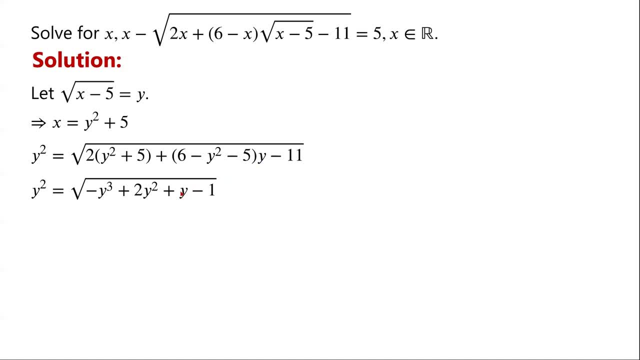 So c squared becomes x squared minus y squared, times 1y squared plus 5y squared, We natürlichi z- инд región. we can write the dogs of r from r, 1 rФ … z goes to. 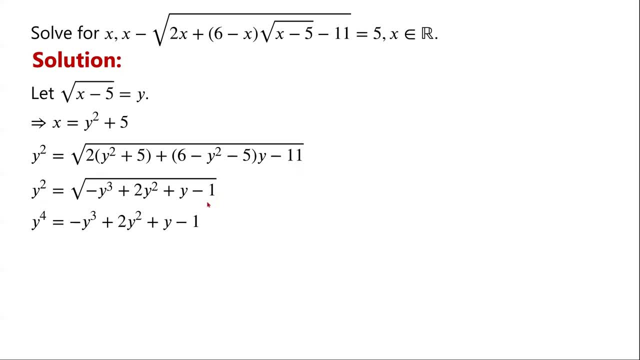 r, 1, rF, U … z go to rf. By integrating the simple algorithm we can also find out that these are growing and sense arrangement values. So y is squared minus Y is 1.. Z minus z equal. minus z is 1 times y. Z is equal minus fights. 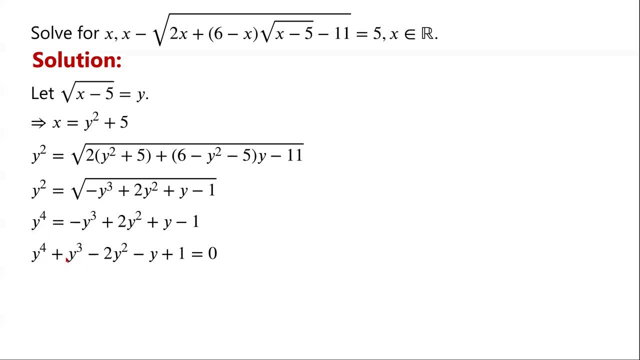 right y to the power of 4 plus y cubed minus 2y squared minus y plus 1 equals 0.. First, two terms have a common factor, y cubed, and they can be written as: y cubed times y plus. 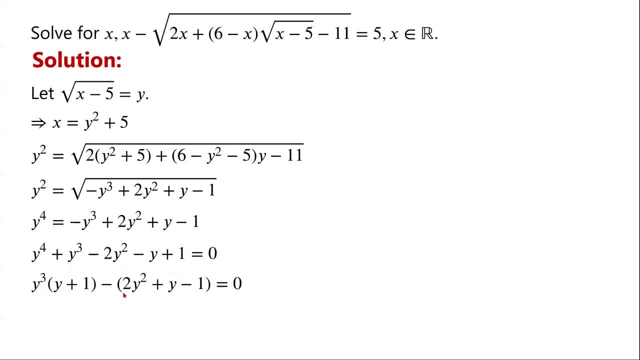 1. The last three terms can be written as minus 2y squared plus y minus 1, which can be factorised and can be written as 2y minus 1 times y plus 1.. We can see that the two terms have a common factor: y plus 1.. 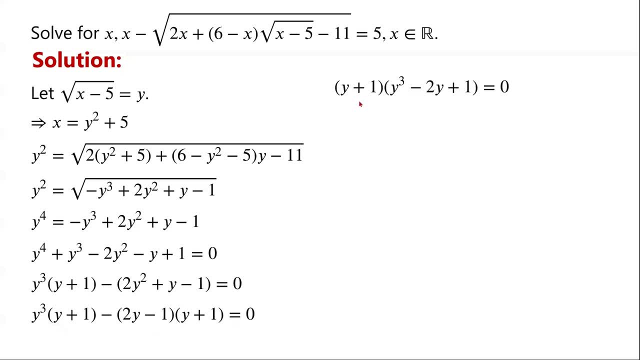 So the equation can be written as: y plus 1 times y cubed minus 2y plus 1 equals 0.. 1 can be written as minus 1 plus 2.. We know that a cubed minus b cubed can be written: 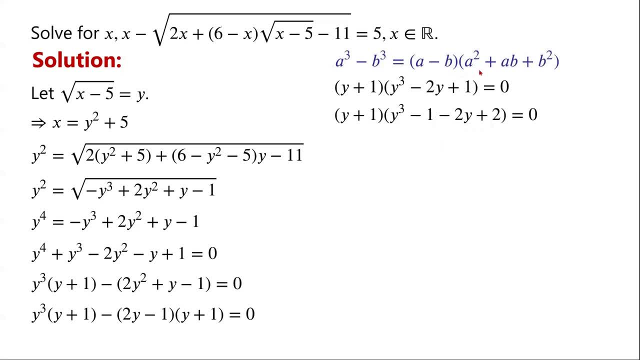 as a minus b. How can we basicly crack out the equation? using a combination of y cubed plus y squared plus y equals 1.. It's the same equation, but we would make sure that y cubed minus y squared plus y plus b. 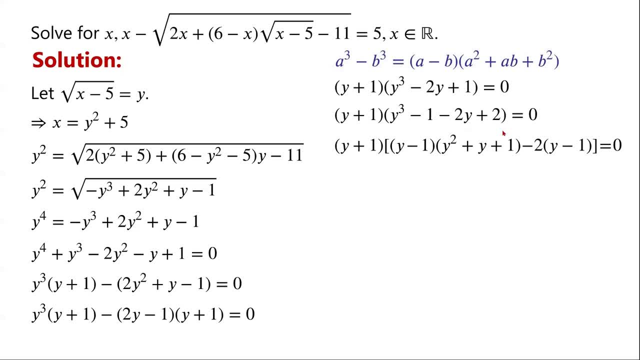 equals 1.. In this equation we need to have a common factor. we simply need to work out a common factor to find out how many squared minus y less than u cubed by multiplying the equation by b, by equalinations and adding up the이에as to' y cubed minus one, which is 1 plus a squared. plus a cubed minus y minus 1 times y squared plus a plus b squared by applying this y cubed minus 1 can be written as y minus 1 times y squared plus y plus 1 minus 2y plus 2 can be: 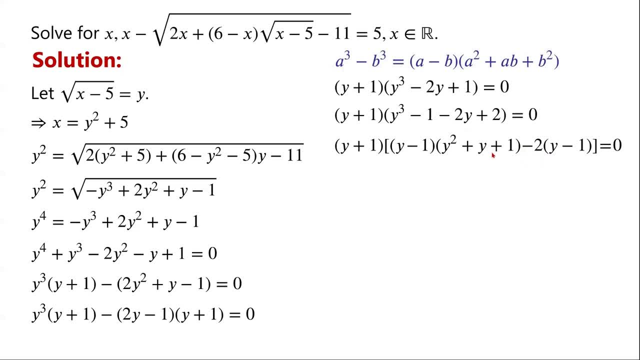 written as: minus 2 times y minus 1 times y, minus one times y squared plus y plus 1 minus cleargasp class cub, and this means Y squared h equals one. We can see that the two terms have a common factor, y-1, so they can be written as y-1 times y squared plus y-1.. 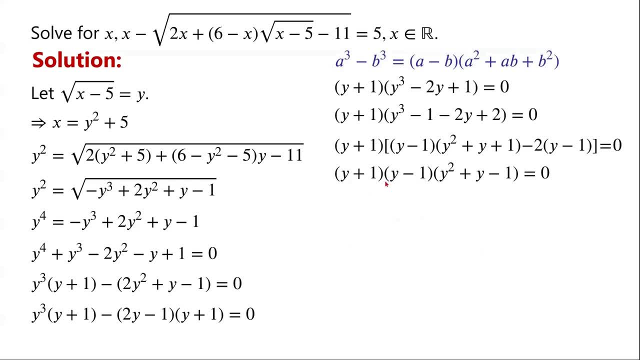 So either y plus 1 equals 0, or y minus 1 equals 0, or y squared plus y minus 1 equals 0. So y1 equals minus 1, y2 equals 1.. By using the quadratic formula: 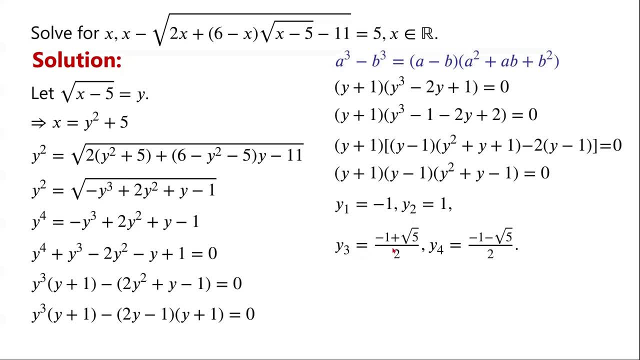 we find that y3 equals minus 1 plus root 5 over 2.. y4 equals minus 1 minus root 5 over 2.. We know that y equals root of x minus 5, which must be root, then, or equal to 0. 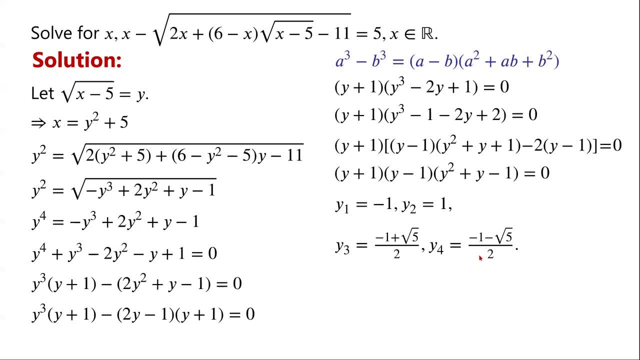 However, y3, y4 is negative, so y4 is discarded as x equals y squared plus 5.. So from y1 equals minus 1, y2 equals 1, x1 equals plus minus 1, all squared plus 5,. 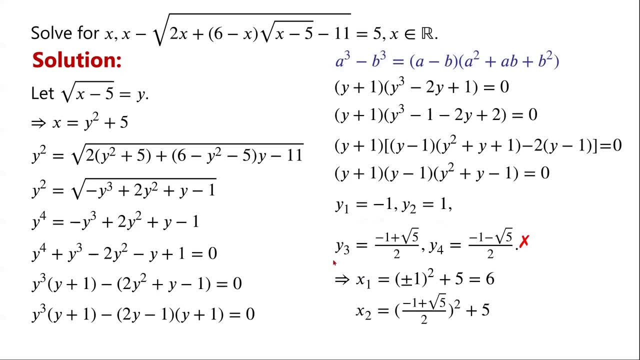 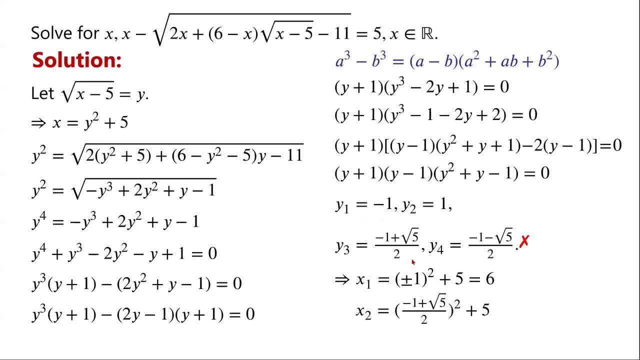 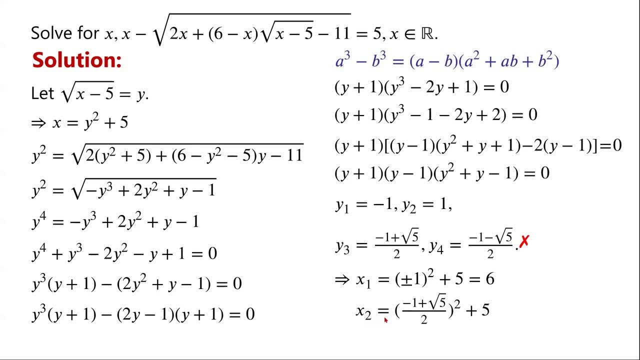 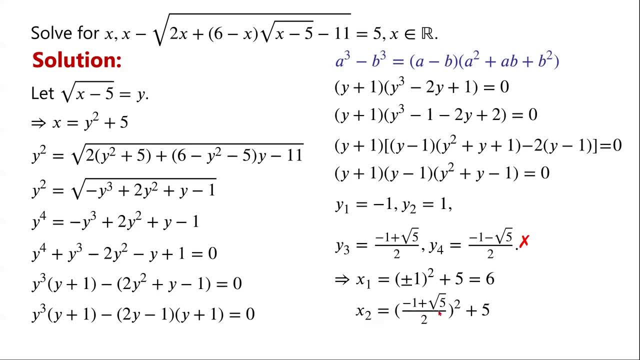 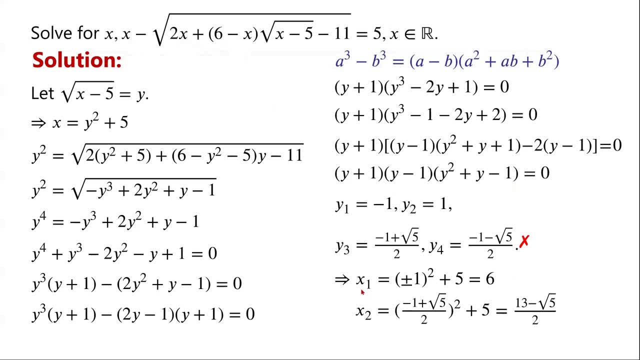 Now we verify whether x1, x2 are solutions of the original equation. If x equals 6, then here we have 6 minus 6, so this term is 0.. 2x minus 11 is 2 times 6 minus 11, which is 12 minus 11,. 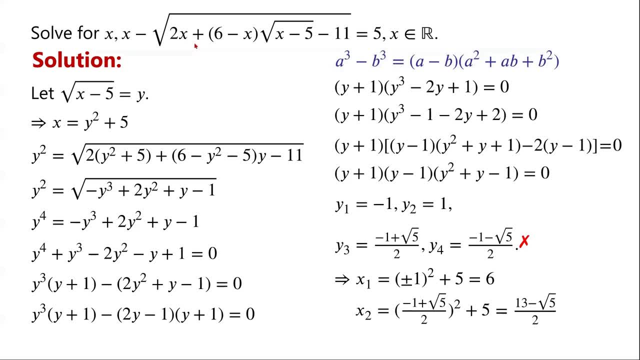 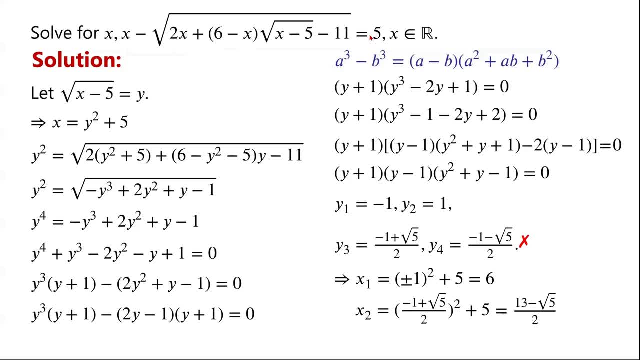 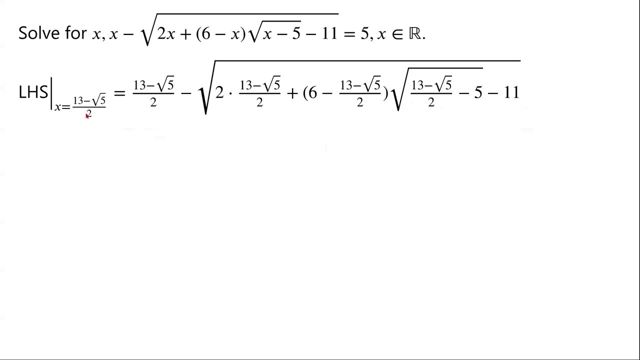 which is equal to the right-hand side of the equation. So x1 equals 6 is a solution of the original equation. Now we substitute: x equals 13 minus root, 5 over 2 in the left-hand side of the equation. 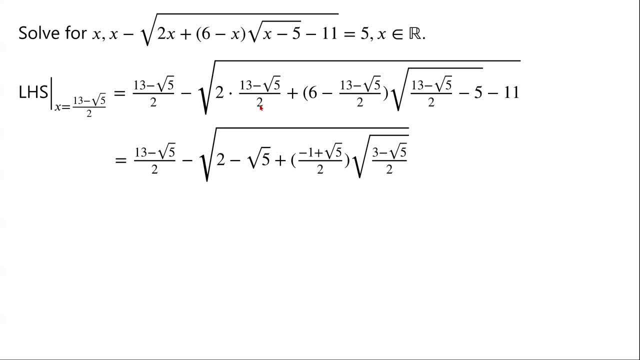 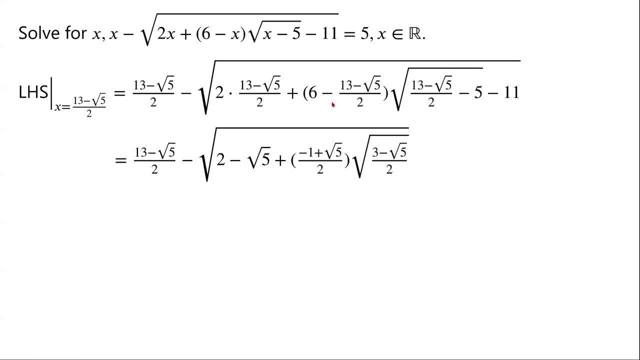 2 here and 2 in the denominator cancel. so we have 13 minus root, 5 minus 11, which is 2.. can be written as 12 over 2.. 12 minus 13 is minus 1.. Minus minus root 5 can be written: 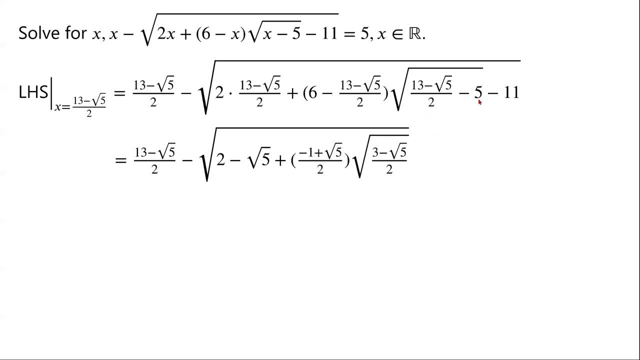 as plus root 5.. Minus 5 can be written as minus 10 over 2.. 13 minus 10 is 3.. Root of 3 minus root 5 over 2 can be written as minus 1 plus root 5 over 2.. 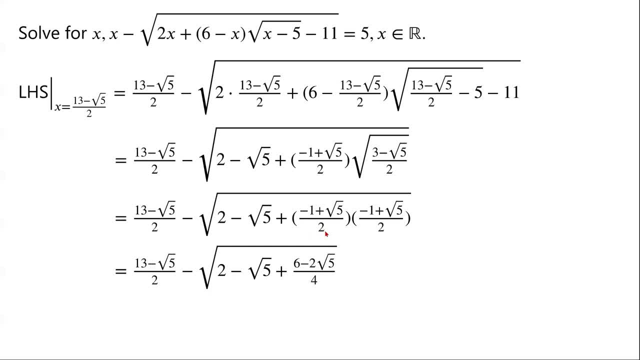 Minus 5 can be written as minus 1 over 2.. 1 plus root 5 over 2, or squared, is equal to 6 minus 2 root 5 over 4.. 6 minus 2 root 5 over 4 can be written as 3 minus root 5 over 2.. 2 minus root 5 can be written as 4 minus 2 root 5. 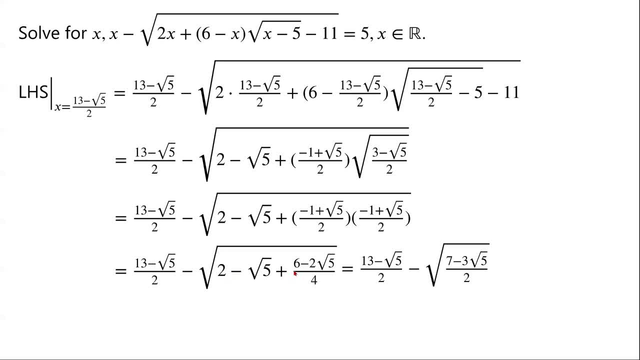 over 2.. 4 plus 3 is 7 minus 2 root 5 minus root 5 is minus root 5 over 2.. 3 minus 3 root 5.. Now we multiply the numerator and the denominator by 2.. 14 minus 6 root 5. 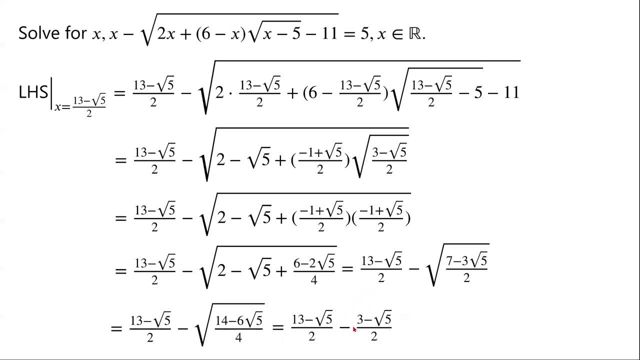 over 4 is equal to 3 minus root, 5 over 2 or squared. So we can now write 13 minus 3 root, 5 over 2 or squared. So we can now write 13 minus 3 root 5 over 2 or squared. 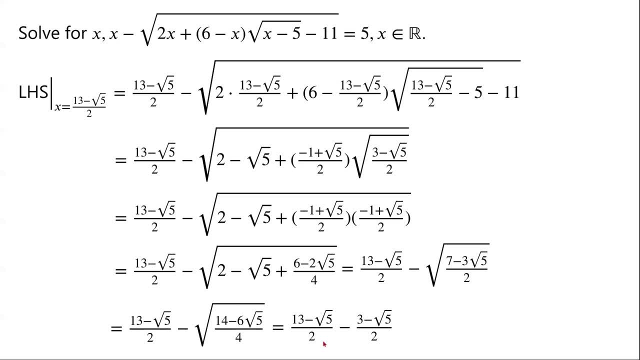